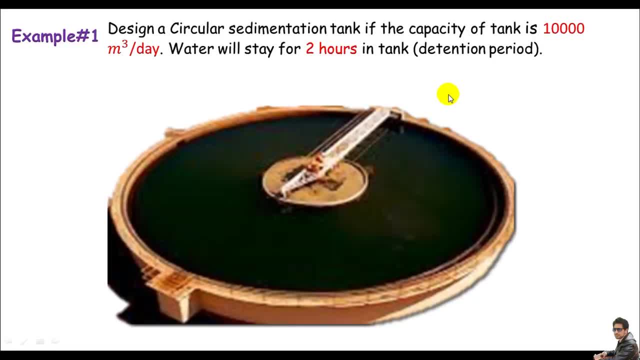 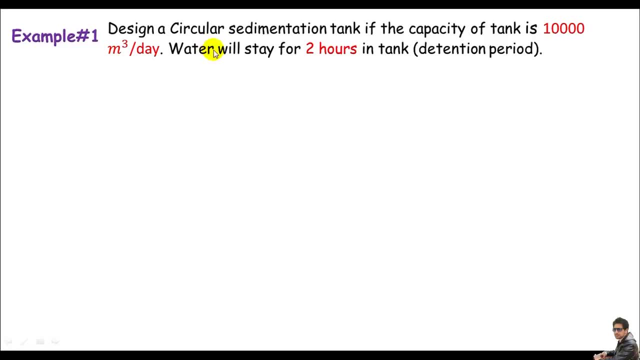 for two hours in the tank. This is also known by detention period. If you see, I think the data is just enough to design the circular sedimentation tank, and here the design means just to determine the diameter and the depth or the height of the tank. 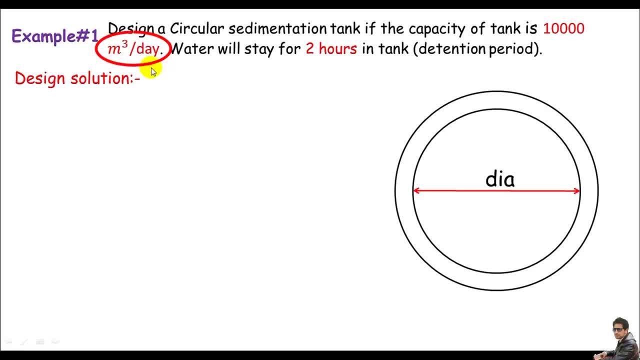 If you see, the tank capacity is just in cubic meter per day. I just need the capacity to gain form of volume and the tank capacity is just 10,000 cubic meter per day. I'll just divide this video by 24, because one day is just 24 hours. If you see, the water will only stay for two hours in. 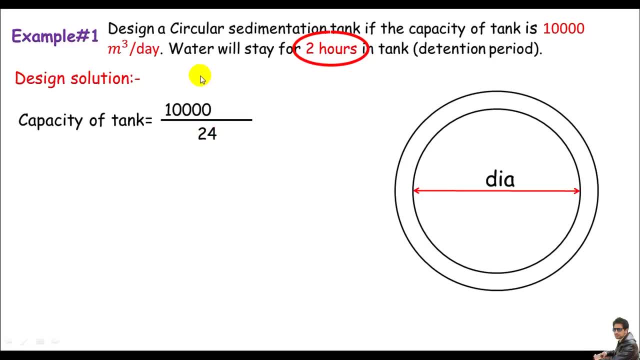 the tank, not for 24 hours or for one day. So I also just involve the specter in this capacity formula. and this is just the point. If the water capacity is 10,000 cubic meter just in 24 hours, how much will be just in two hours? 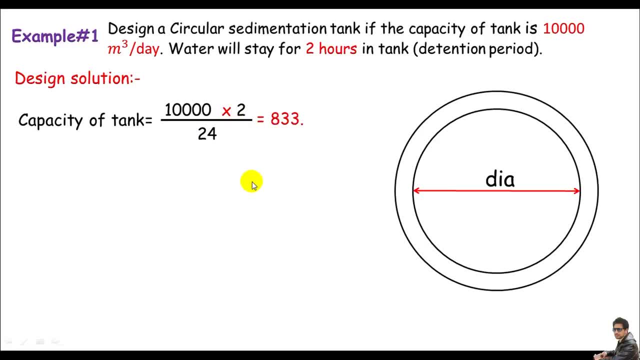 So do some plug and chug and you'll get, of course, 8334, and 34 cubic meter is the capacity of given tank. Now, this is just in form of volume, right, and the volume of circular sedimentation tank may be just in this form. the area of the base stands the height, Because this is just a 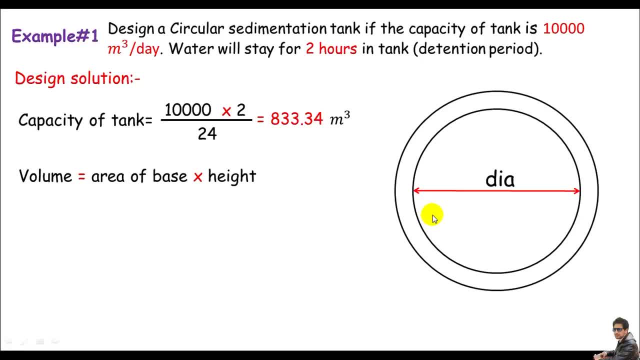 cylinder, a circular cylinder? a hollow cylinder maybe? okay, and the volume. remember the area of the base. this is just a circular base, all right. this is a circular sedimentation tank. so the area of the base will be just pi d squared divided by four, or just pi r squared, no problem, you can. 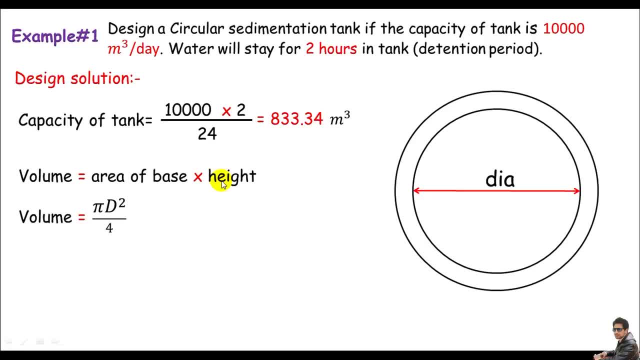 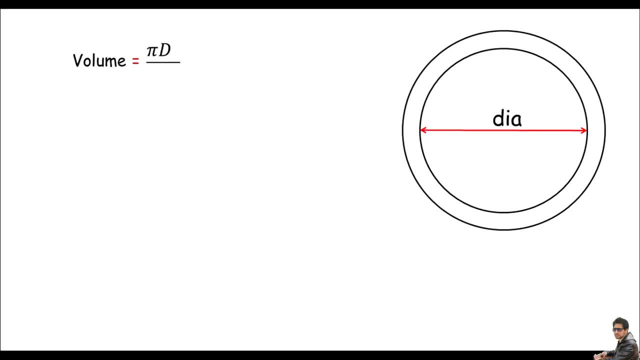 use one in these formulas: times the height or the depth. I don't have many rooms in this page, so let me start a new page. The volume is pi d squared divided by four d squared divided by four times the height. If you see, the diameter is unknown, the height is also. 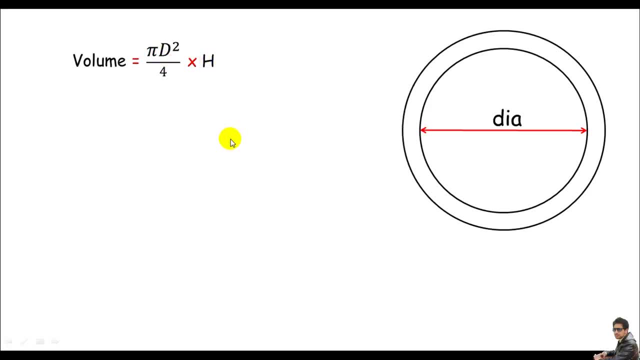 unknown, so we should assume one thing. Let's assume the height or the depth is just three meter. This is a nice assumption, No problem. if you design your tank and the diameter is just a not good value, you can of course change your assumption and review your design. This will depend upon your site. For this time, let's 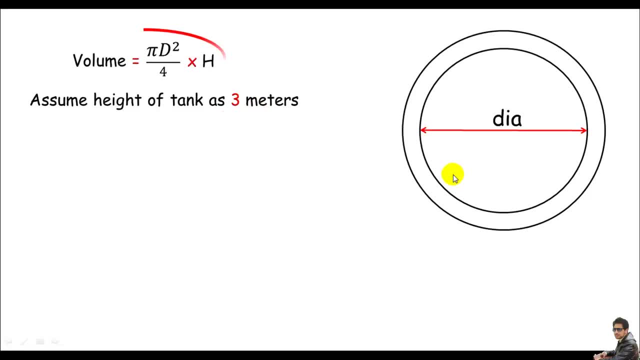 try three meter as the height of the tank, and let me put this video in this formula. Remember, the volume is given, which is of course 833.34 cubic meter. we did this guy a few minutes ago. The diameter is unknown. so pi d squared divided by four times the height, The height is just three meter. 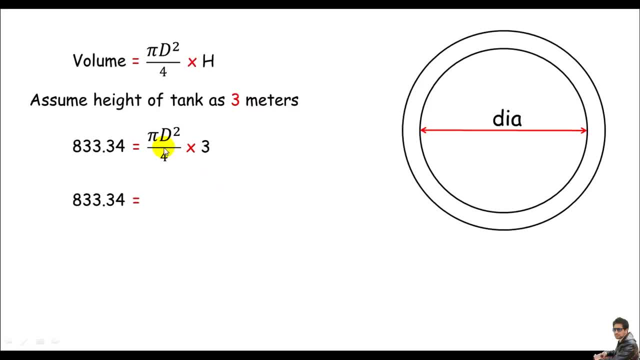 If you do some short maths like three times pi divided by four, this is of course 2.356 and d squared. If we divide both sides by 2.356, we can get, of course, d squared equals 3, 5, 3.68.. 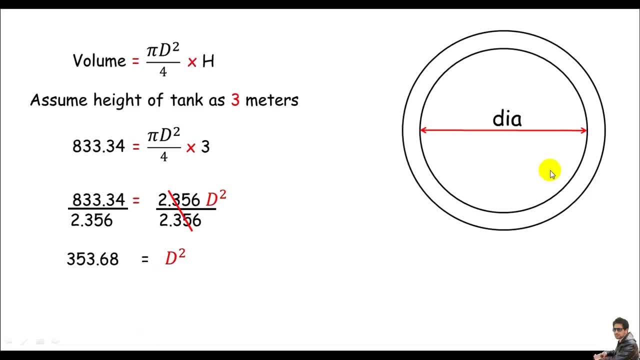 Remember, we only need d, which is just the diameter of sedimentation tank. So we just need to put square roots on both sides. We can get. of course, d equals 18.8 meter. Let me just assume or say the diameter is just 19 meter, because 18.8 meter is just of. 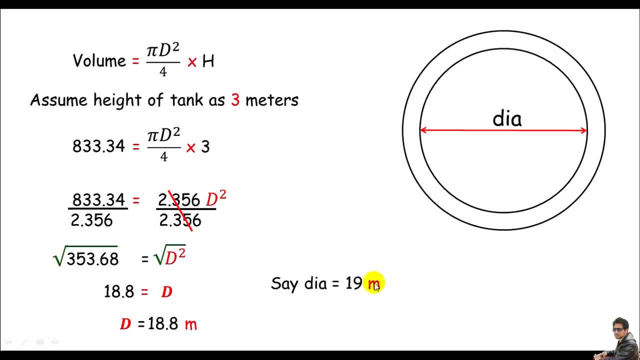 course the same value as 19 meter. This is just so adjacent to 19. okay, Only just 20 centimeter is just the difference, no problem. So I think 19 meter is a better value per diameter. okay, If 19 meter is not suitable for your site, I mean if you don't have much site. 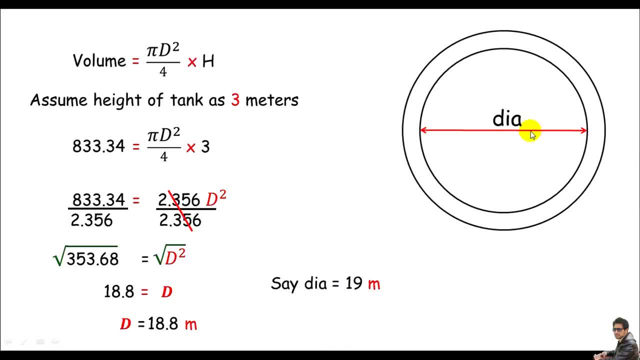 per 19 meter as the diameter of the tank. of course you can just increase the depth of the height of this tank. Of course your diameter will decrease gradually In short term if your site is not good for 19 meter, as the diameter of the given sedimentation tank, just increase. 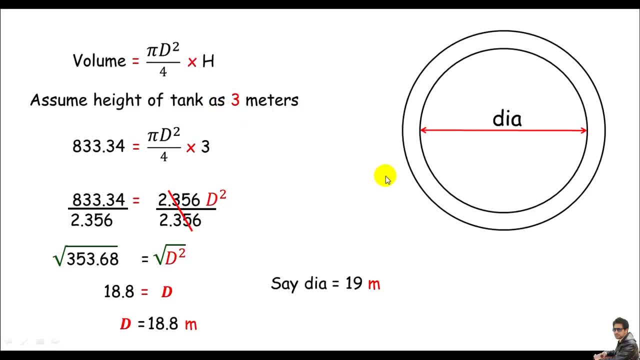 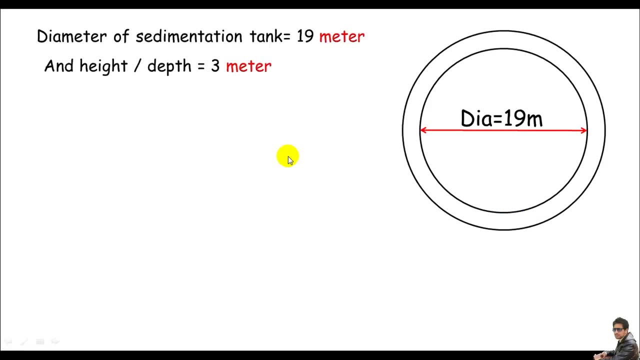 the depth or the height of the tank. Of course, 19 meter, which is the diameter, will come down. So we got a nice video for diameter of the tank, which is 19 meter. Remember, the depth or the height of the given tank is just three meter and this was just our assumption. Let me just 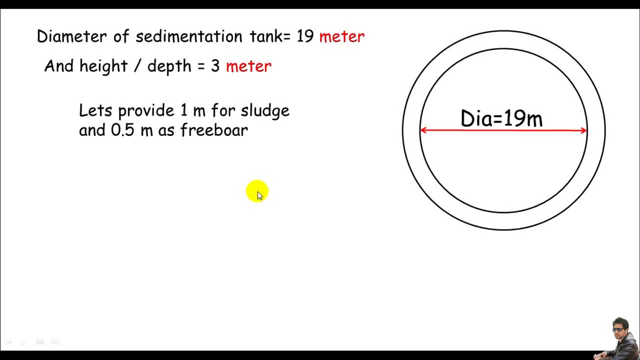 provide one meter per sludge and 0.5 meter is pre-board, So the total depth must be 3 meter plus 1 meter plus 0.5 meter. This is, of course, 4.5 meter, And this is it. of course. We have done it.